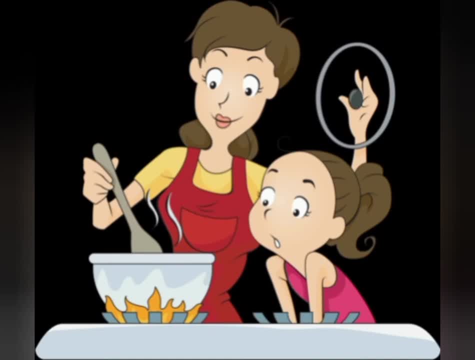 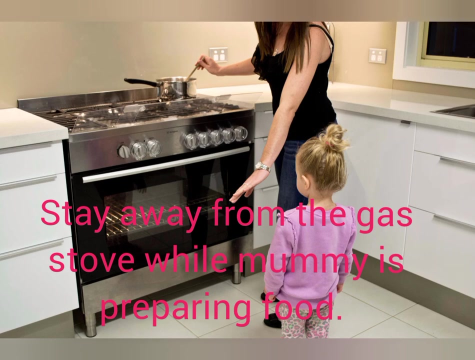 Don't leave it open. Do not disturb your parents or your mama while she is cooking. It's very dangerous to disturb Anyone while they are cooking or while they are near the fire or the gas stove. Always stay away from the gas stove, from the fire, while your mommy is preparing food. 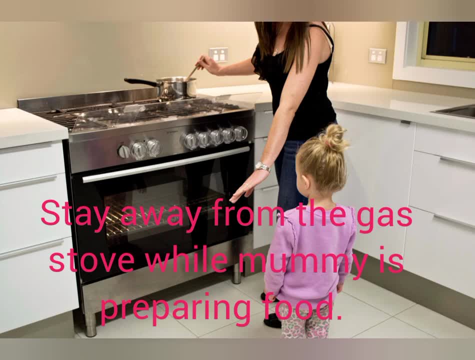 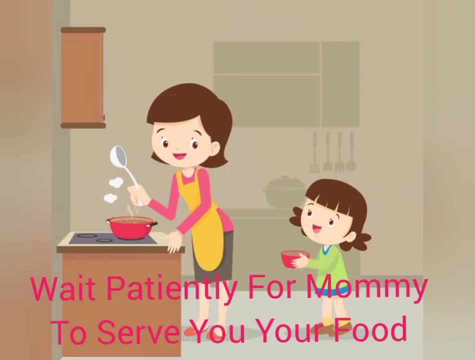 Do not come near the gas or the gas stove. Do not come near the fire. Please stay away from it. Okay, You must also wait patiently for your mommy to serve you your food. Okay, Don't disturb. Don't keep on disturbing your mama while she is cooking. 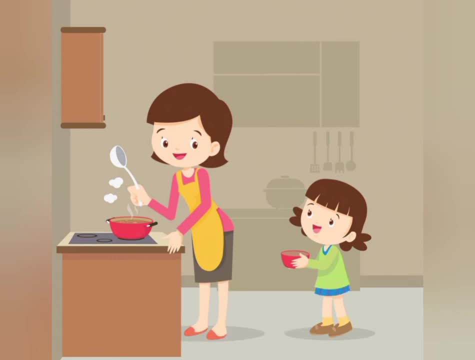 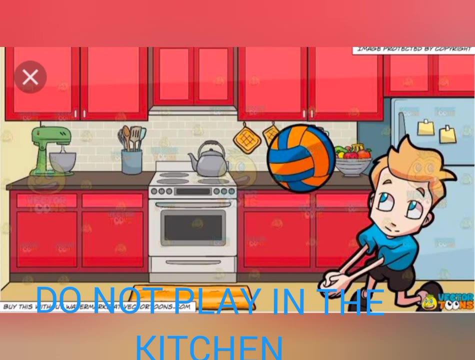 Simply wait patiently for your mom to serve you the food. Do not play in the kitchen. Yes, children, Kitchen is not the place to play, Right? You should always play in the playground Outside, So do not play in the kitchen. 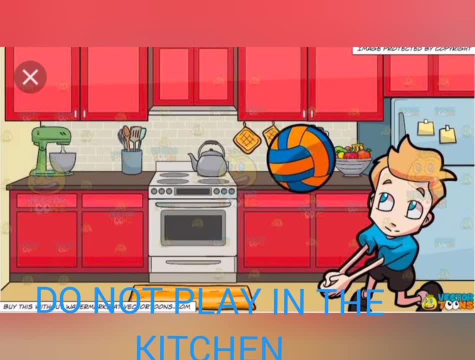 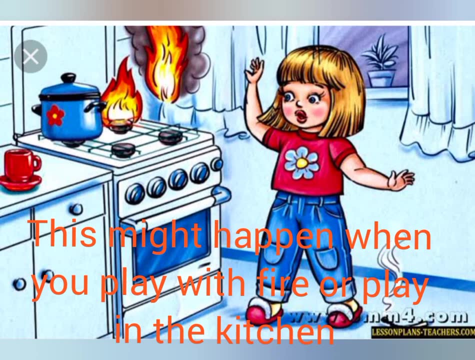 Never do that. Na na na, Never do that. And do you know what will happen if you play in the kitchen? Yes, this might happen. Right, Are you afraid of the fire? Look? So you should keep away from the fire and also not play in the kitchen. 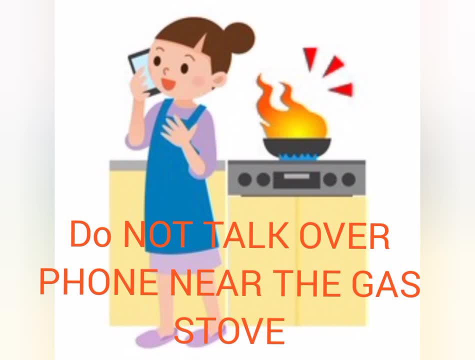 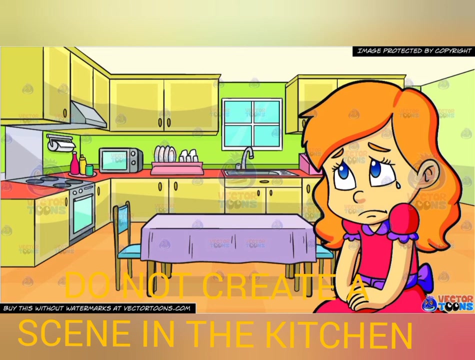 Another thing: do not talk over the phone near the gas stove or near the fire. You should not use the phone when you are cooking or when your mama is cooking. You should keep away your phone while cooking near the gas stove or fire. Do not create any scene in the kitchen. 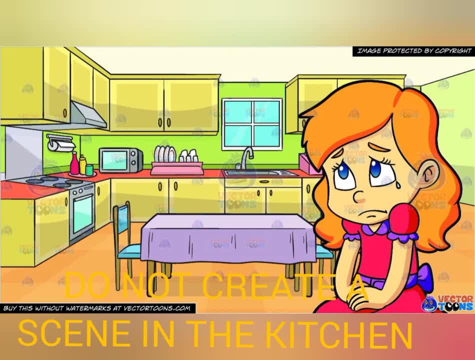 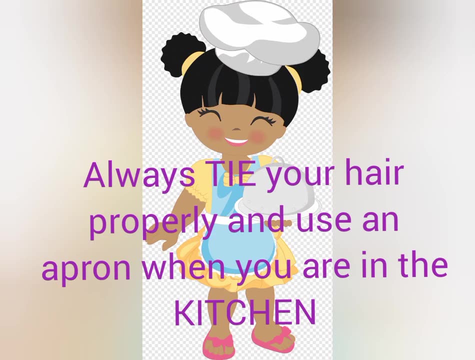 Most children love to ask something or disturb the phone, Or disturb or cry in front of the parents, Isn't it? But do not do that in kitchen. This could be dangerous, Then what else? Always tie your hair properly and use an apron when you are in the kitchen.